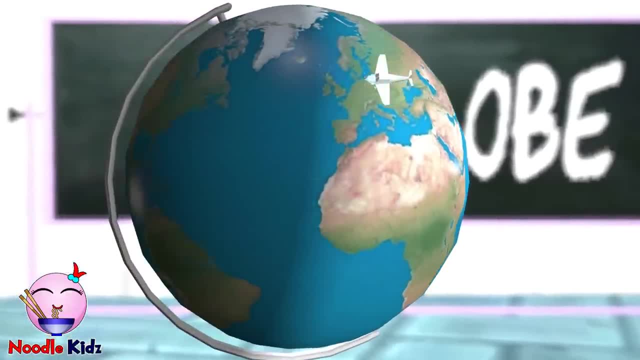 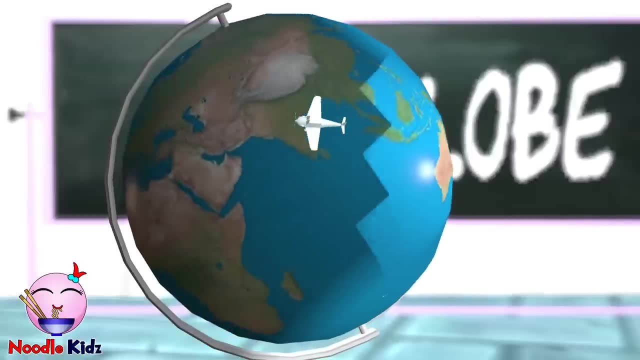 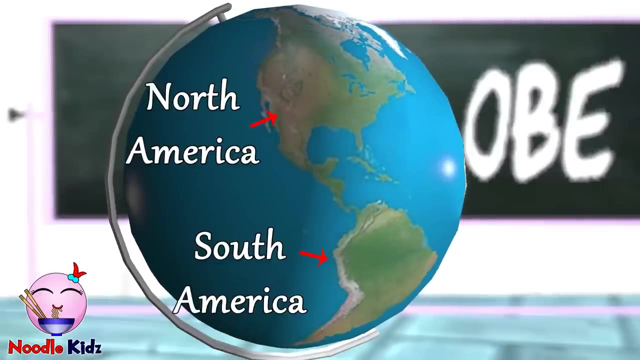 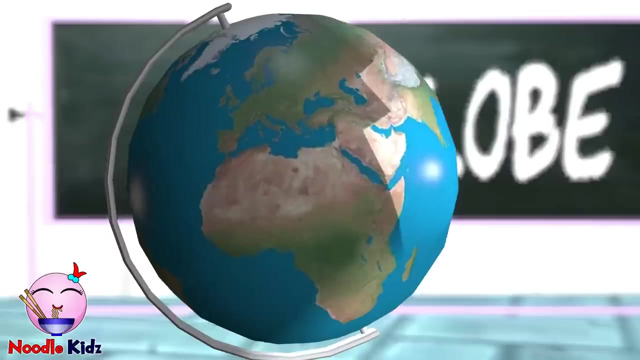 time. You can also simulate a flight from one place to another place through different routes and show that our earth is round. You can rotate the globe and see the continents of the world. Here you can see North America and South America. This is Africa, Europe. 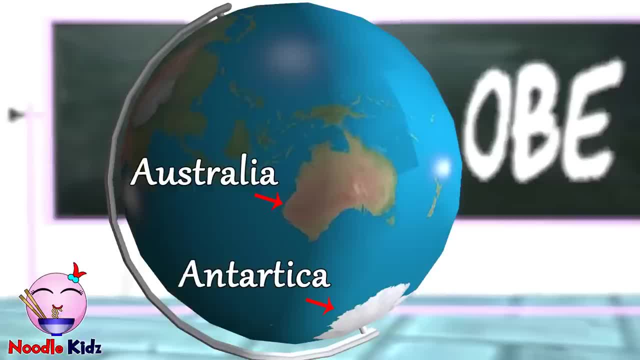 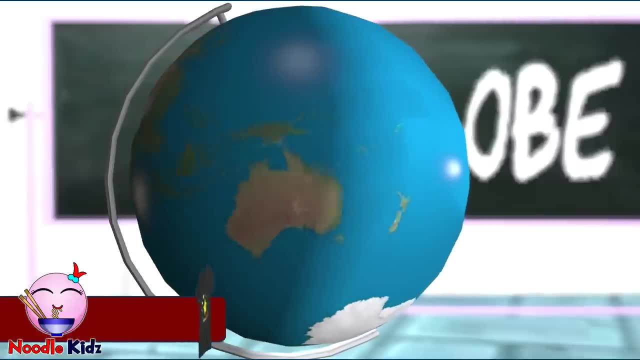 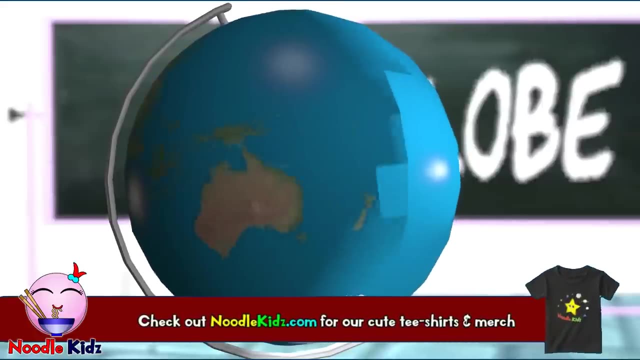 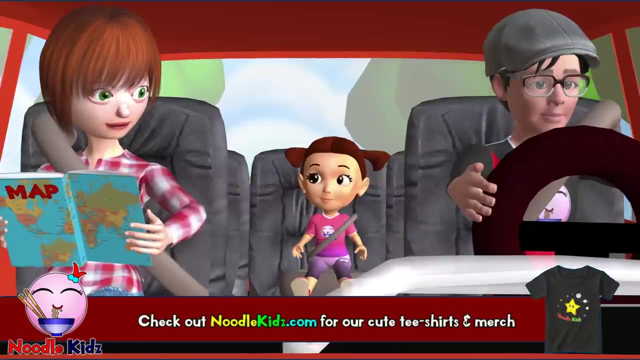 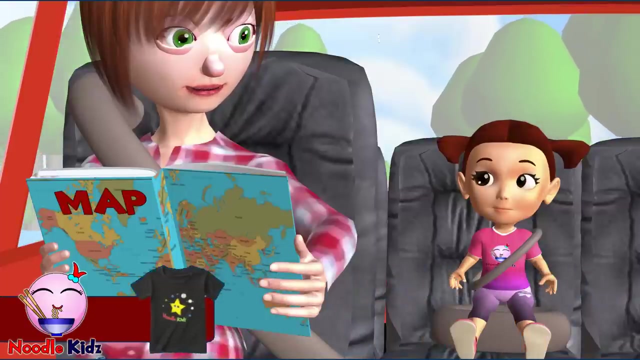 Asia, Australia, and and and and. A globe can be called as a duplicate Earth. It is round in shape and shows more accurate areas, distances, directions and relative shape and size. Then what's a map? A map gives a two-dimensional presentation of certain regions in the world, and you can 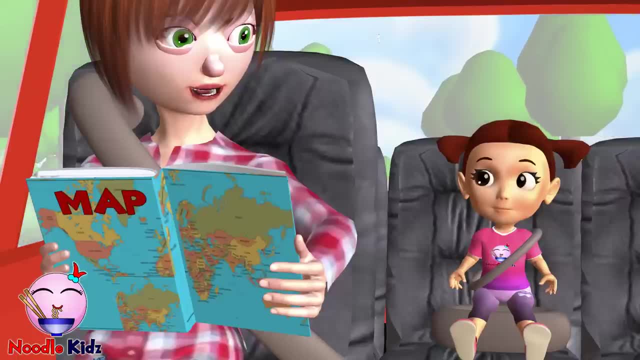 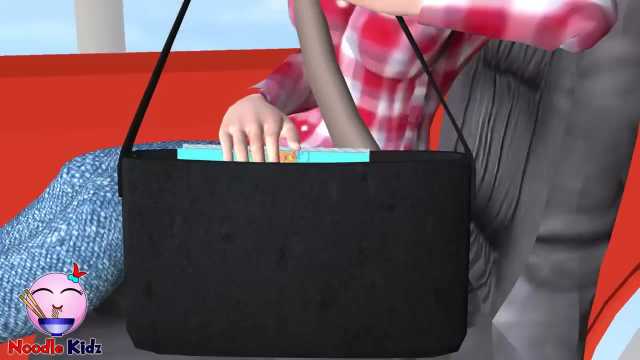 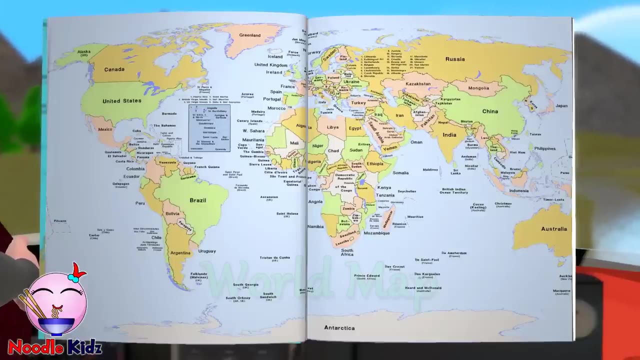 see this map is in Mommy's hand. It is easier to use and portable. I can easily put this map in my purse and bring it wherever I want. There are many kinds of maps. This is a world map which shows the continents and countries in the world. 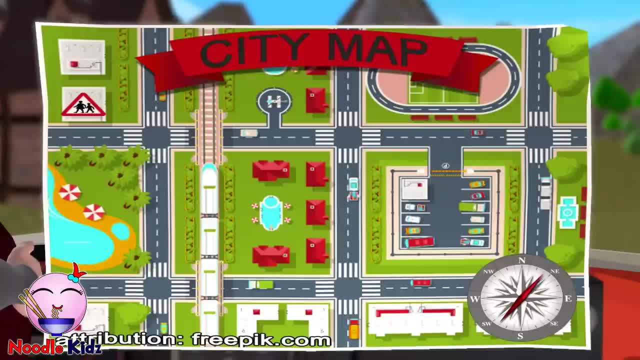 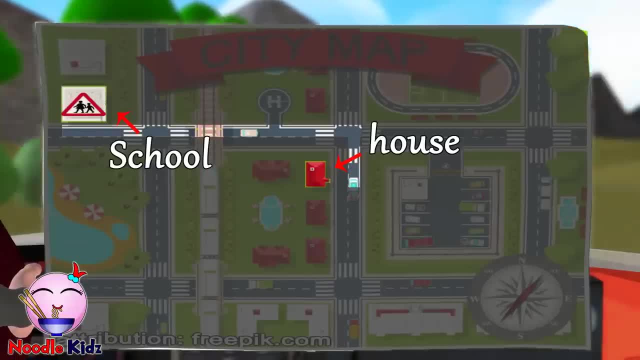 This is our city map. This is our city map. This is our city map, which shows the roads, parks and public places. See, That's your school And our house is here. With this map, we know how to get to school from our house. 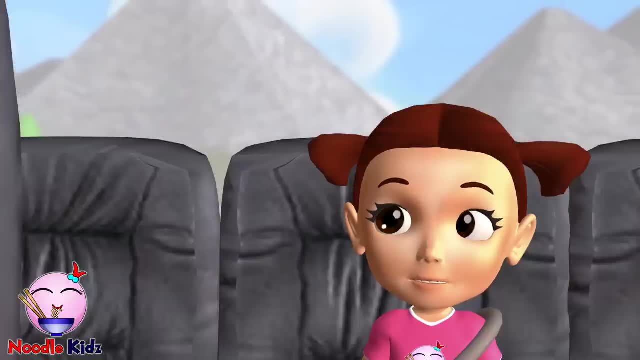 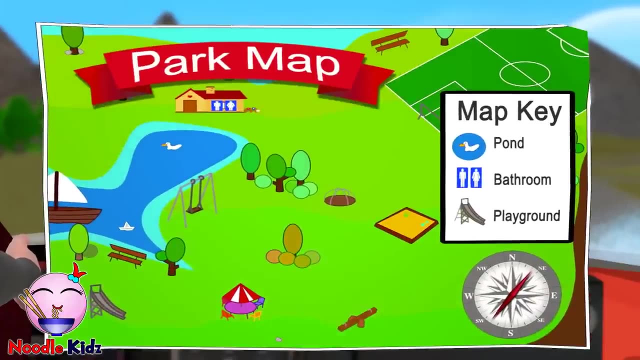 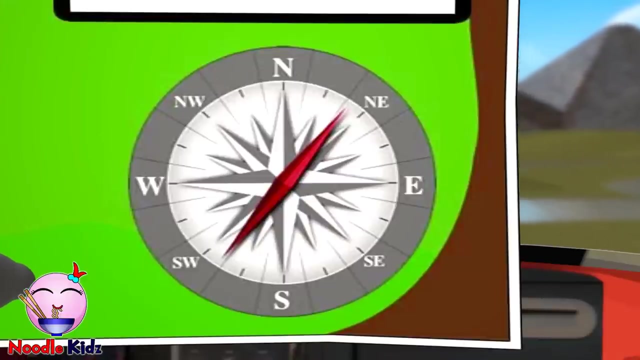 Wow, that's really helpful. And this is the park map. It shows where the play areas are, the walking paths and the park And the bathrooms. Wow, that's really helpful. And what's this? This is a compass rose. 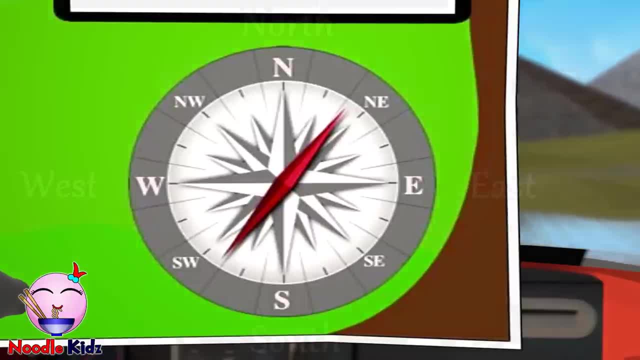 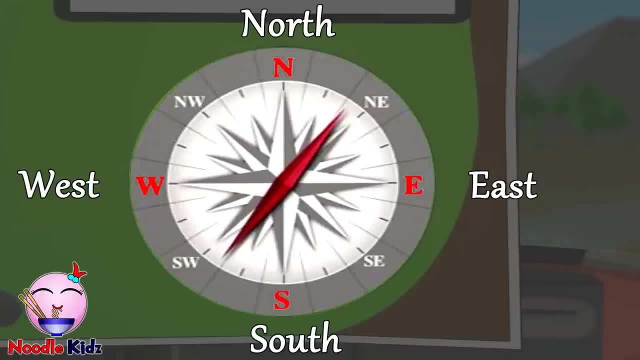 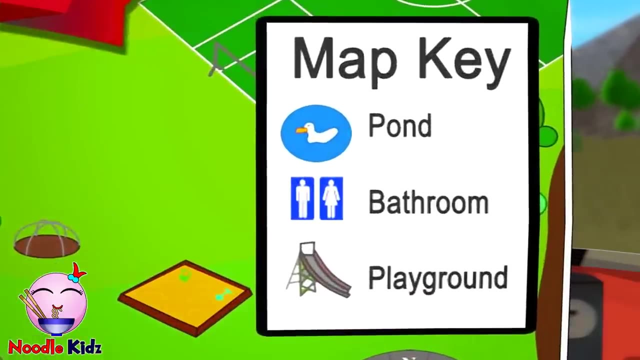 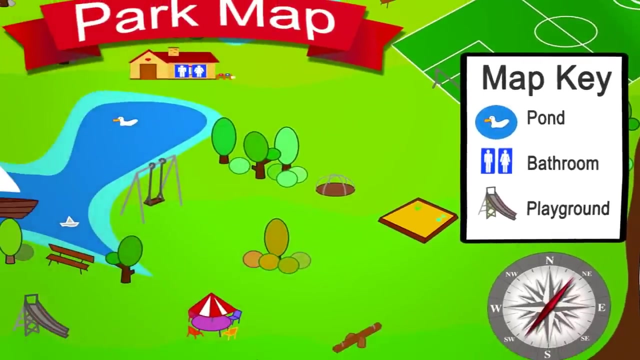 It's used to display the orientation of the directions: N is for North, S is for South, E is for East And W is for West. And what are these symbols? This is the map table key. It helps us identify what's on the map. This way, we can find what we're looking for.